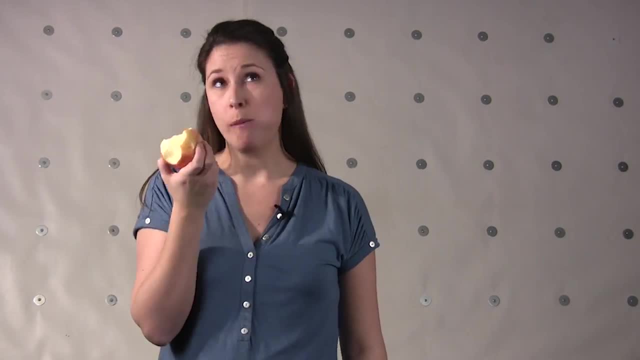 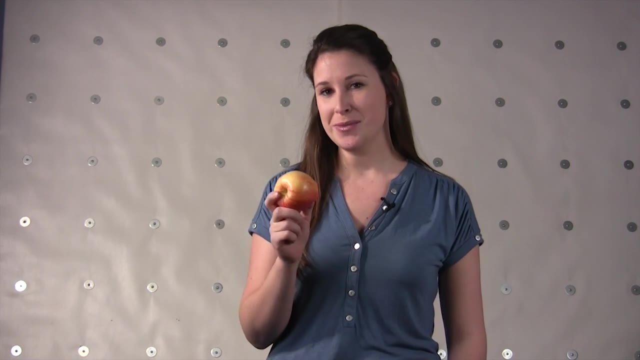 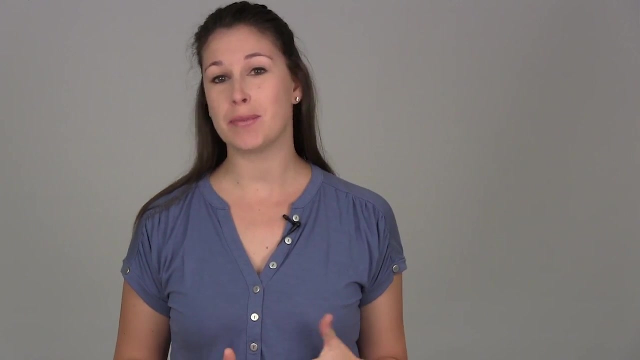 apples with even more energy, Just like me. nuclear power plants need fuel to keep them running, but they use something a little more potent than apples. At Canadian Nuclear Laboratories, researchers and engineers are working on fabricating new types of nuclear fuels. every day, A nuclear 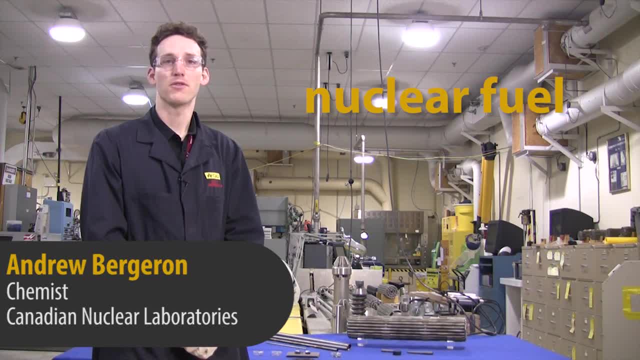 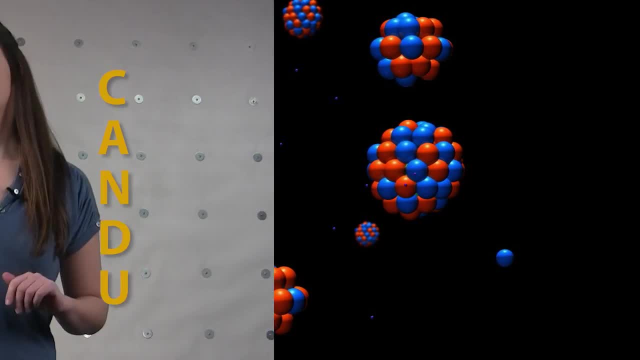 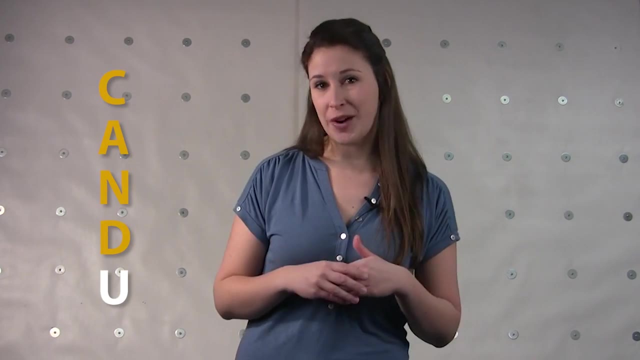 fuel is a material that produces heat through fission. Fission is a process where an atom is split apart, producing energy in a nuclear reaction. CANDU reactors produce all nuclear energy in Canada using deuterium oxide, also called heavy water, and natural uranium. The uranium is used to produce a nuclear fuel which is called deuterium oxide. The uranium is used to produce deuterium oxide, also called heavy water and natural uranium. The uranium is used to produce deuterium oxide, also called heavy water and natural uranium. The uranium. 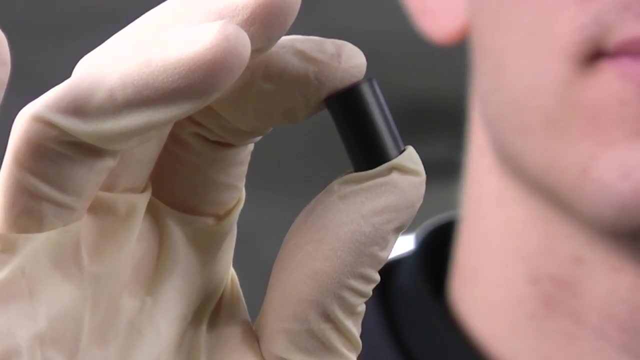 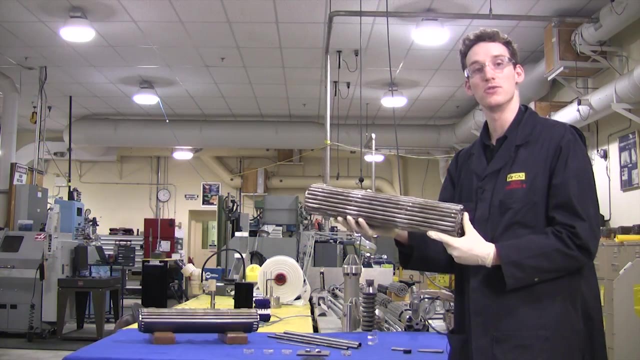 is what fuels the reactor itself. compacted into pellets and placed into a fuel bundle- This is a nuclear fuel bundle that's used in a CANDU reactor. This fuel bundle goes into a fuel channel in a nuclear reactor and the fuel bundle produces heat. This fuel 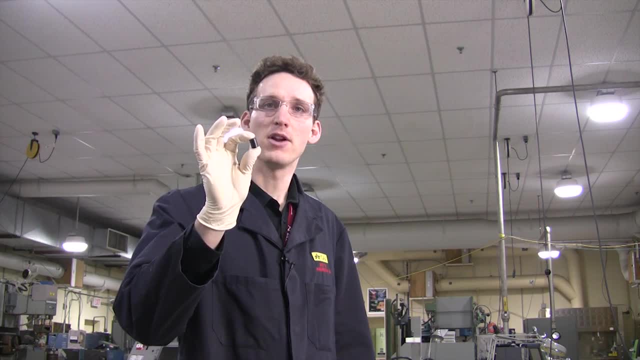 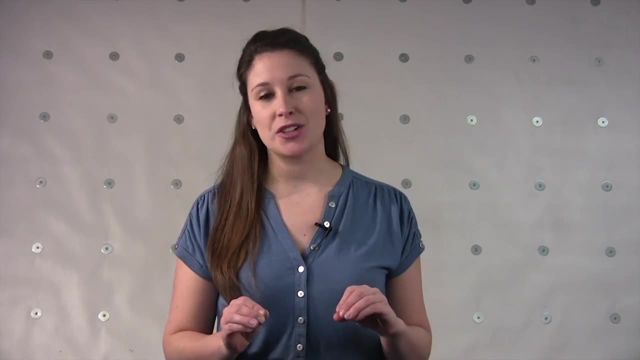 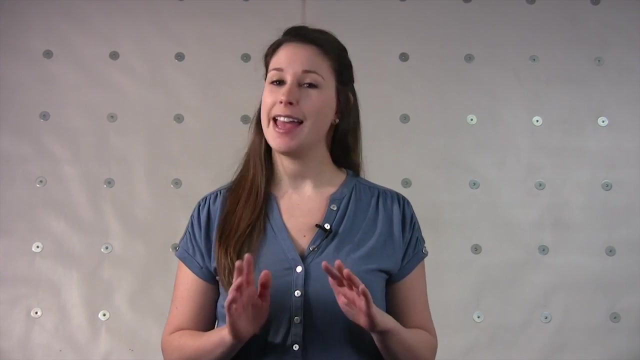 pellet is incredibly energy dense. It has the same energy content as thousands of barrels of oil or tons of coal. The fuel inside a CANDU reactor can last anywhere from one to two years before it's removed. The spent fuel has to be handled very carefully because it's hot. 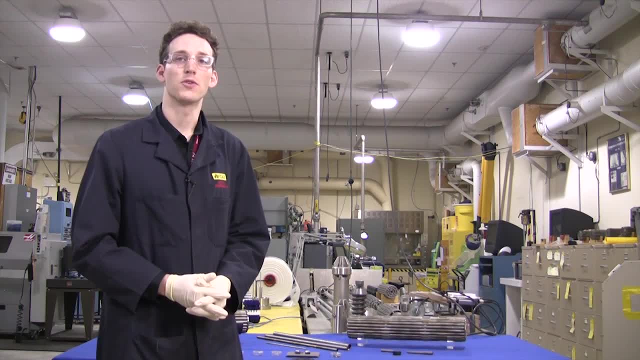 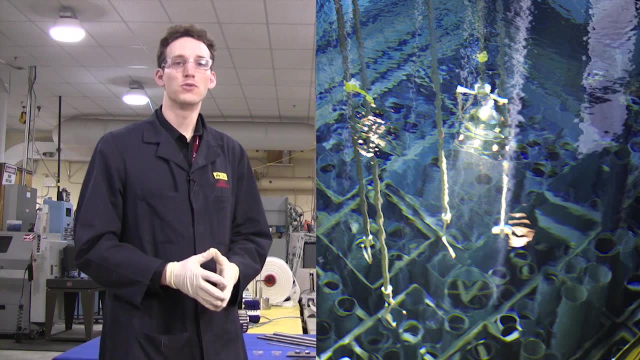 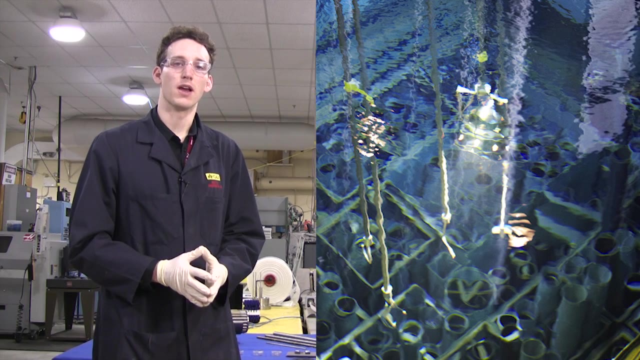 and radioactive. When the used fuel is discharged from the reactor, it goes to spent fuel cooling bays which are filled with water. The water serves to cool the fuel after it's come out of the reactor because it's still quite hot, and it also serves as a radiation shield for the 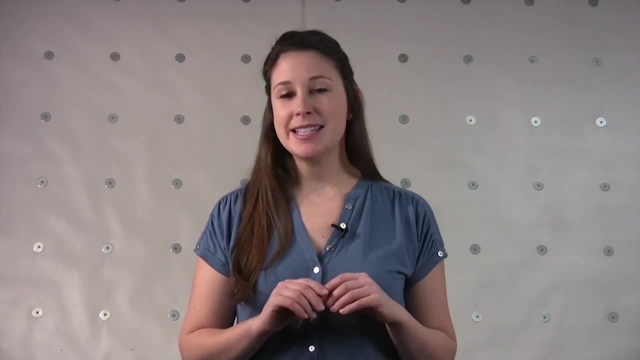 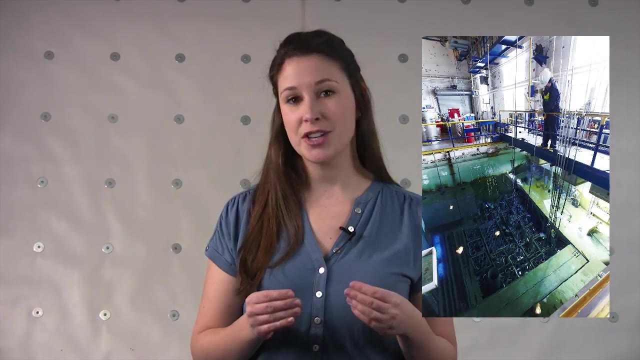 radiation coming off the used fuel. This spent fuel stays in the cooling bays for a minimum of ten years before it's removed. It's then stored in a dry storage facility where concrete is used to shield the leftover radiation from the rest of the environment. 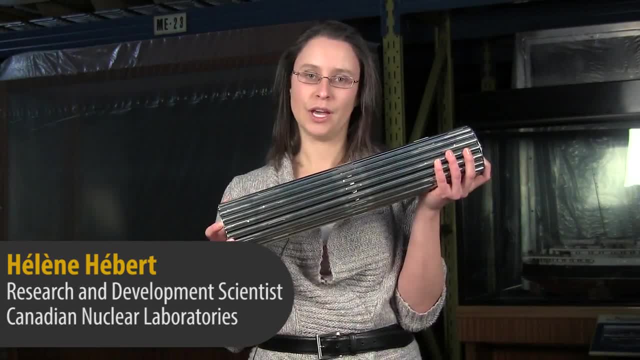 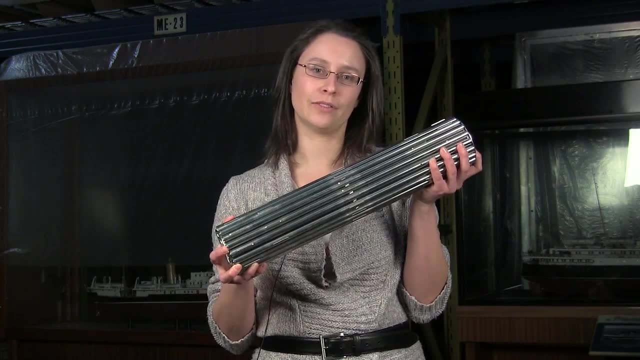 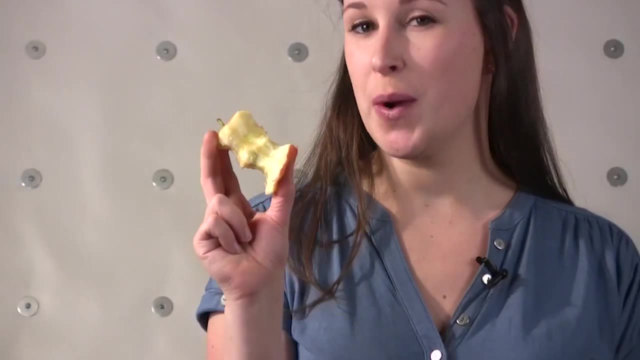 You can see that once this fuel bundle has been used, it doesn't go into the atmosphere. It's in solid form. This is what we have to deal with. It's compact and it's a small footprint. But what if we could choose compost recycling over the waste bin for spent nuclear fuels?